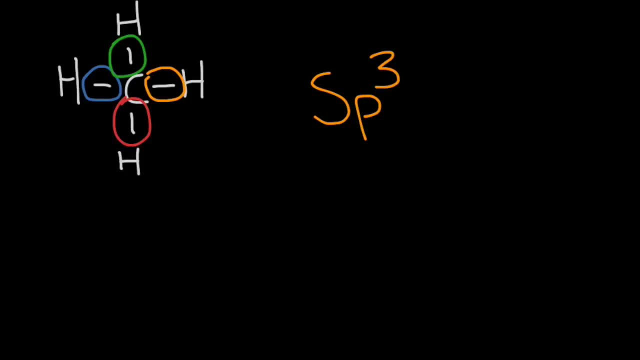 And, like we said, each single bond represents one point. Let's try another one. Our next one has a carbon attached to it, One oxygen and two hydrogens. So let's take a look. We'll circle this double bond And, as always, a double bond is going to count as one point, the same as a single bond. 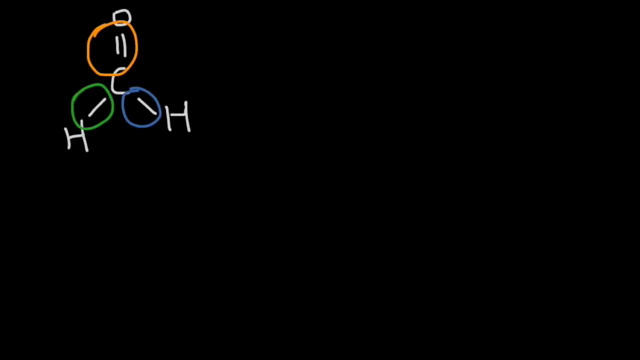 There's another one And there's our third one, attached to that last hydrogen. So we have three values, three points, And if we have three points, we know that we have a hybridization of sp2.. Our next one: There's a beryllium attached to two fluorines. 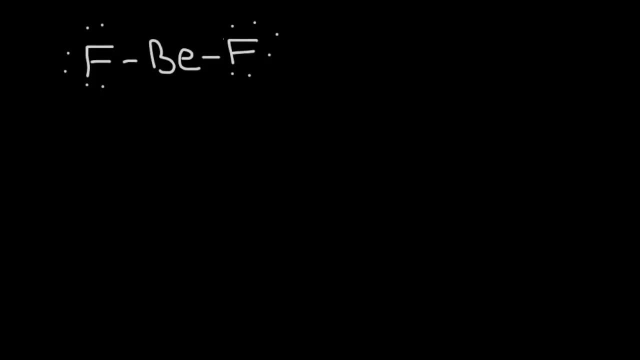 So let's look at what's around here. So what you might do- and this might be a mistake that some of you may make- is you might consider circling these lone pairs, And actually that would be incorrect, because we just have to look at what's around the beryllium. 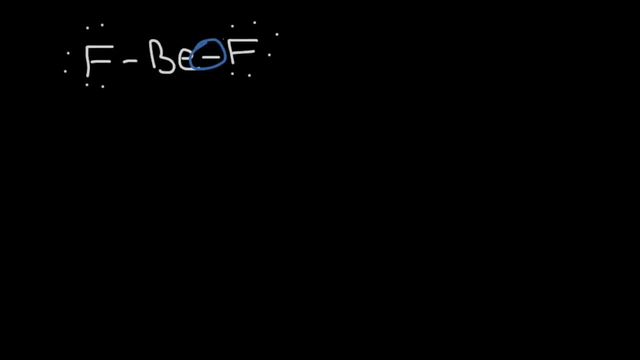 So we just have to look at the central atom, because that's what we're trying to determine. the hybridization of. So beryllium only has a steric value of two, So it has two points. So the hybridization is going to be sp. 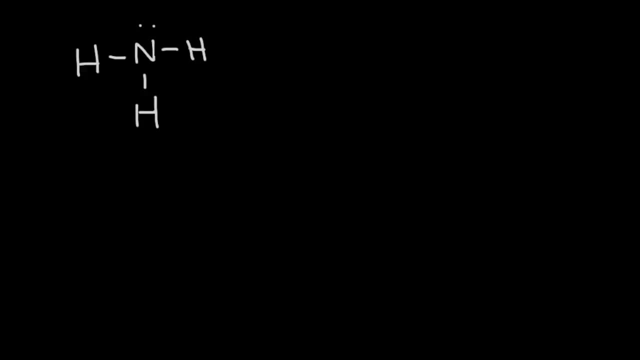 Our next one is a nitrogen bonded to three hydrogens and has a lone pair on it. Now, this one for the lone pair, you actually will count it because it's attached to the central atom, which is the nitrogen. So one, two, three, four. 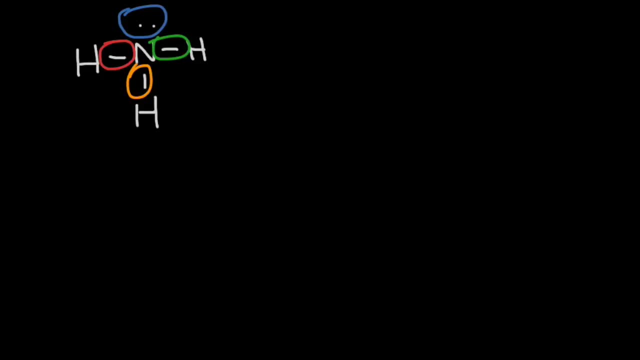 Once again, we have a steric value of four and that means we will have a hybridization of sp3.. So, to recap, a single bond, a double bond, a triple bond and a lone pair of electrons, all of those equal one point. 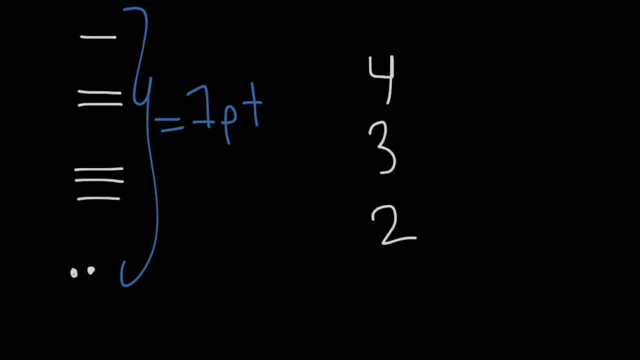 All of them stand for one point. Be sure to remember that, because it's important. And if we have four points, that means we have a hybridization of sp3.. If we have three points, sp2.. And two points is just sp. 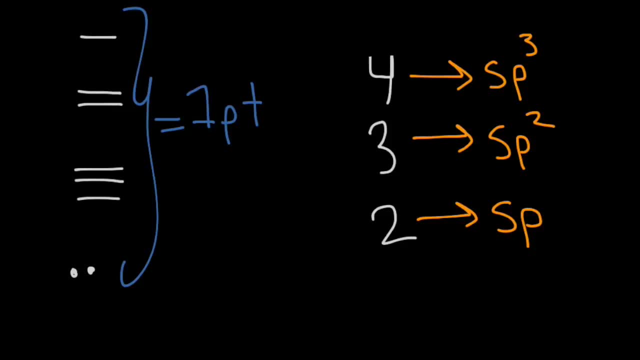 Thank you guys for watching. If you have any questions, please feel free to leave them below in the comments.